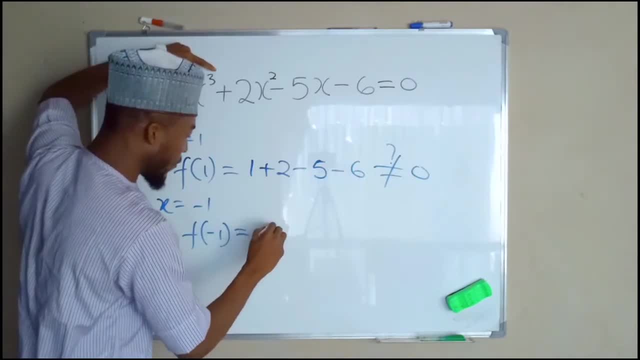 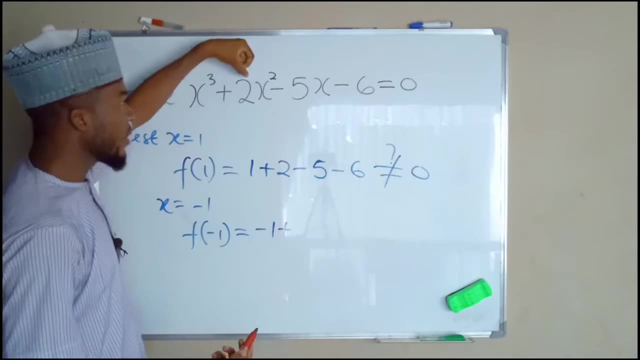 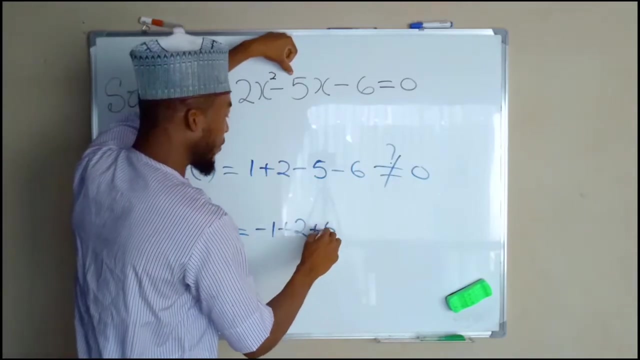 negative 1 to the power of 3 is still negative. 1 plus negative 1 to the power of 2 is positive. 1 times 2 is 2.. Negative 1 times negative: 5 is positive 5.. Then minus the constant, If this: 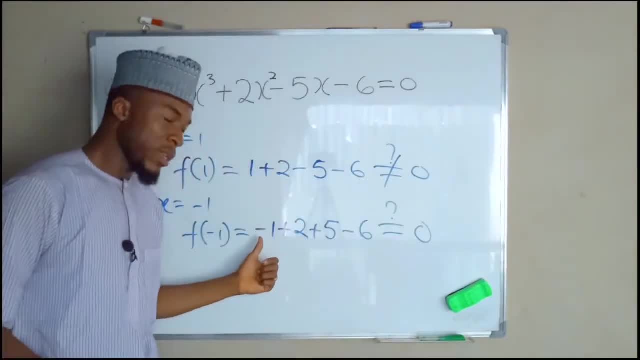 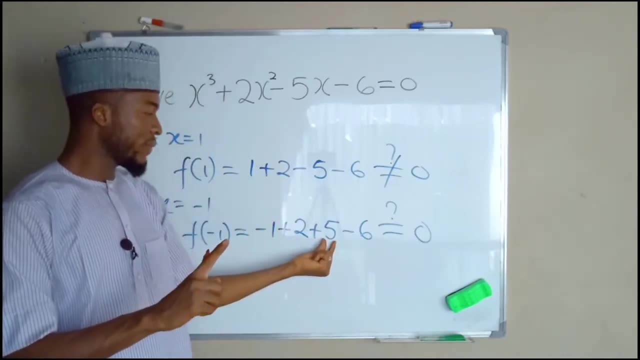 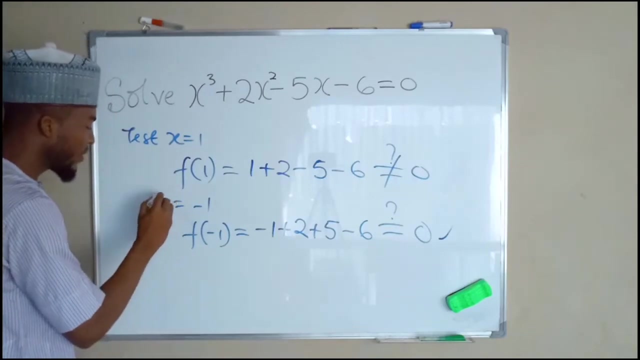 is equal to 0.. All right, Negative 1, positive 2 is positive 1.. Positive 1 plus 5 is positive 6.. 6 minus 6 is 0. Therefore this satisfy the equation. Hence we say: negative 1 is one of. 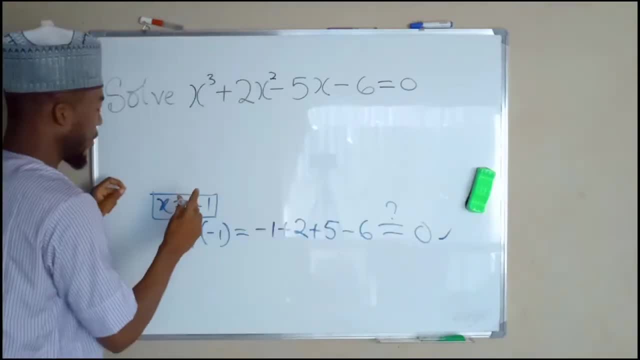 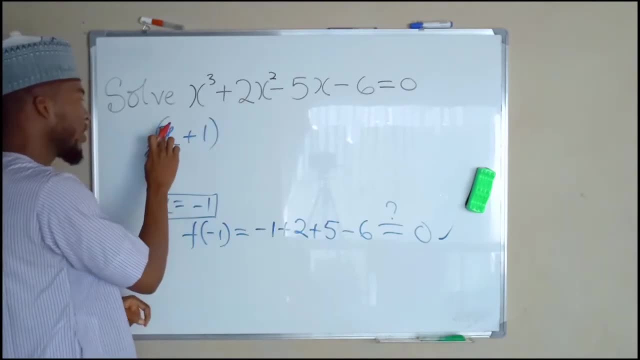 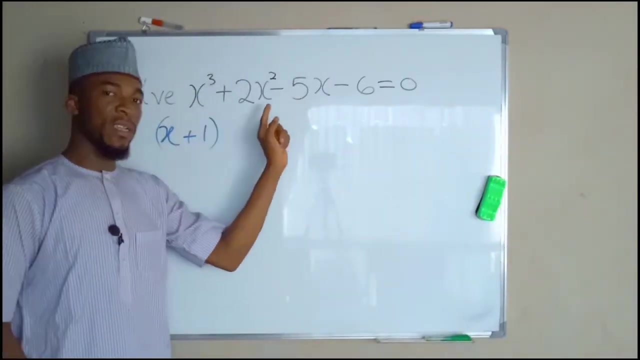 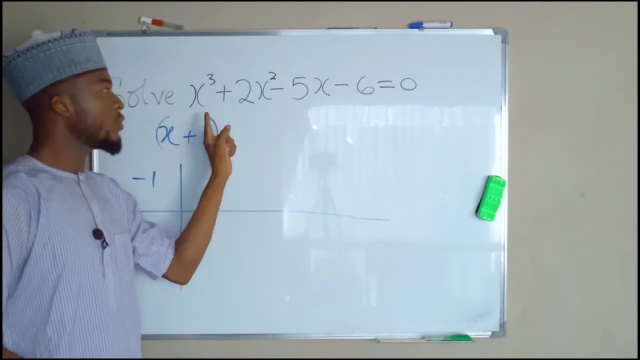 the roots of this cubic equation. Therefore, x plus 1 is one of the factors of this cubic equation. So let me show you how we are going to find the other factors. Already we have seen that negative 1 satisfy this equation, So we have our negative 1. here We are going to write down the coefficient. 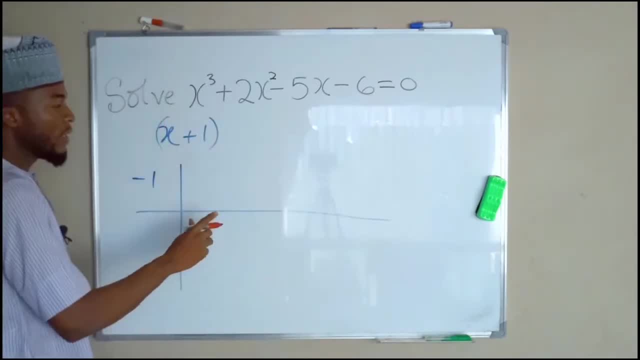 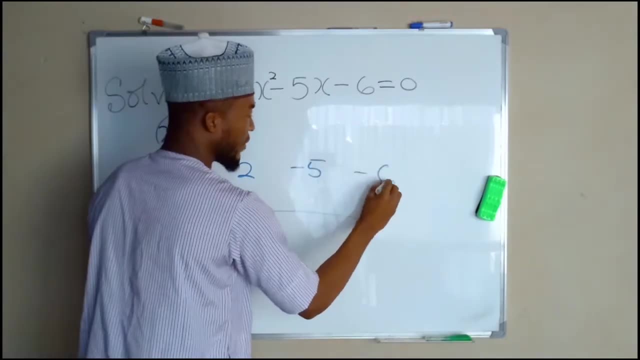 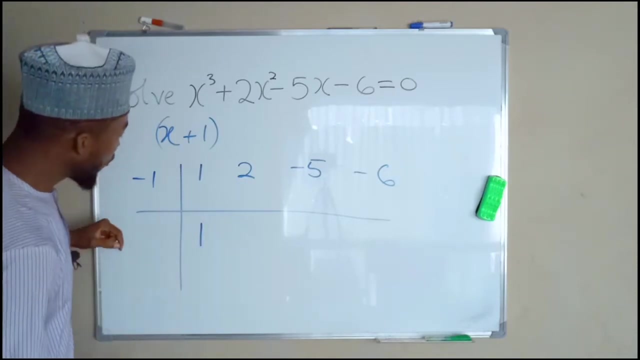 of this cubic equation, including the constant term, The leading coefficient is 1,, 2,, negative 5, and negative 6.. We are going to drop down the leading coefficient, which is 1.. So now what we are going to do. we are going to multiply this negative 1 with this positive 1.. 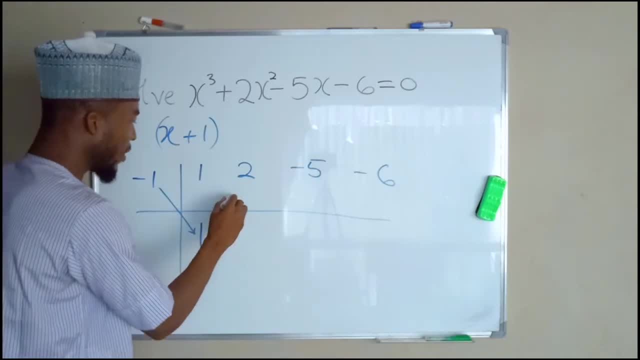 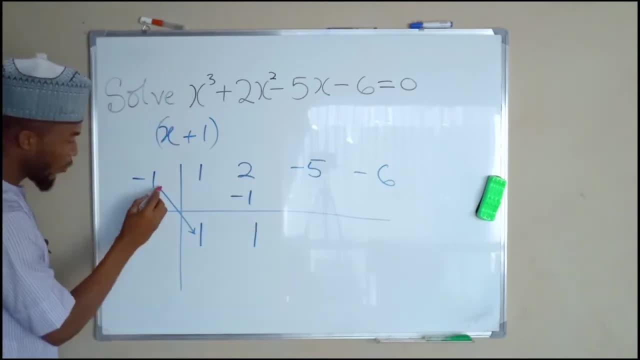 Negative 1 times positive. 1 is negative 1. Then we write it here. Then we add these two together: This plus this is positive 1. We multiply this again with this positive 1. This time this is negative 1. We write it here on that negative 5.. This plus this is negative 6.. 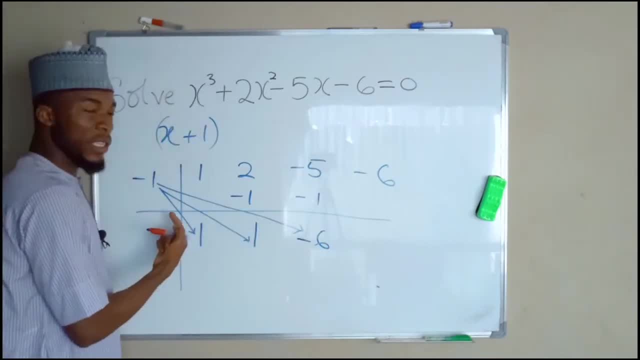 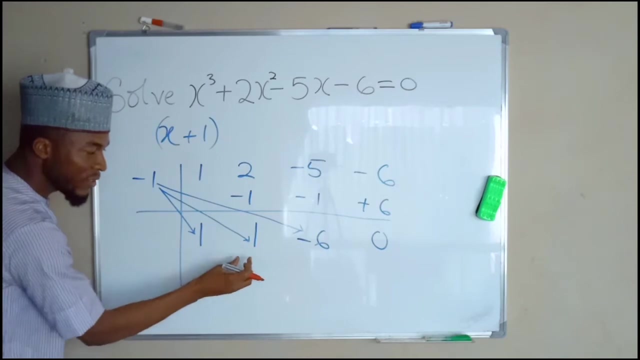 Again, we multiply this with that negative 6 and it will give us positive 6.. If you add this together, you get 0. Hence we are going to form a quadratic equation using these constant terms. This is the leading coefficient, This is the coefficient of the middle term and this is the constant term.